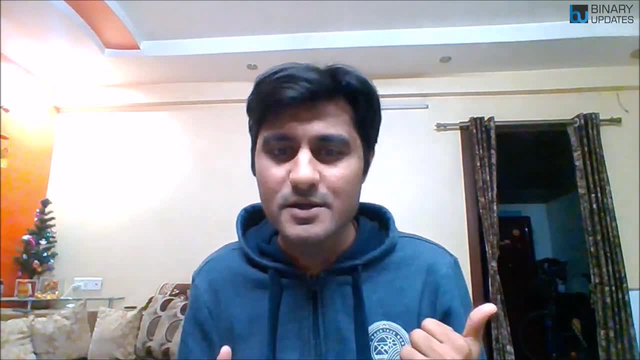 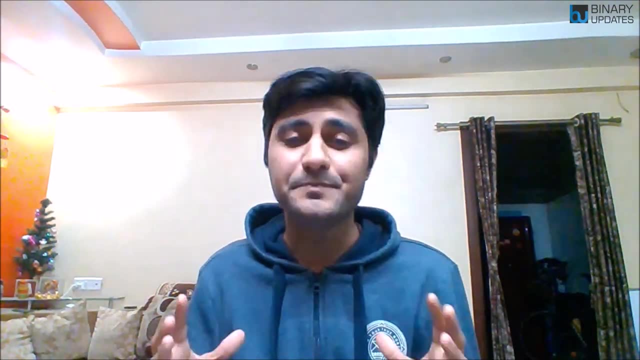 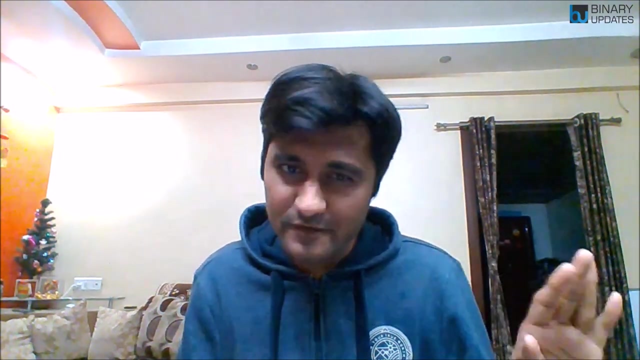 I worked with a lot of companies. I work for healthcare, I work for PCB manufacturing company and I had my own startup, and right now I'm a founder of binary updates, calm. So if you really want to make the career as an embedded system engineer, Then you could either look out for embedded hardware development. 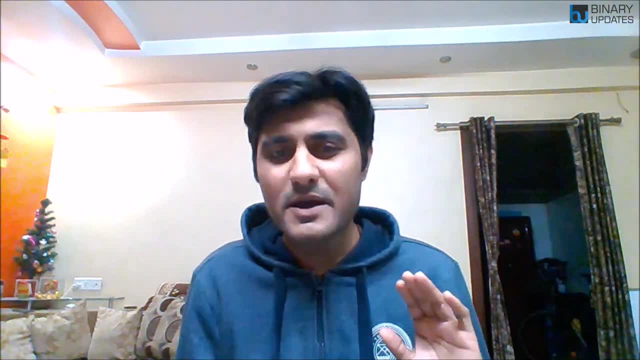 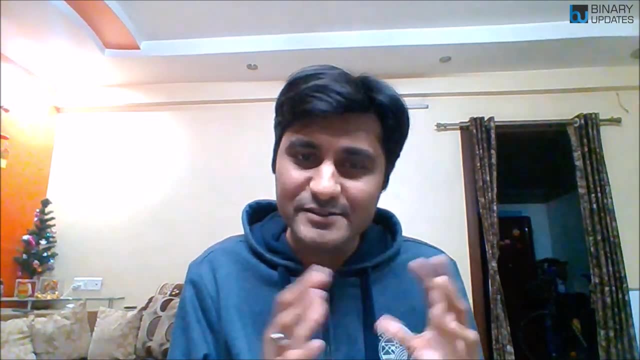 The other part is embedded software development. if you want to prepare for embedded hardware engineer, Then you might have to be look out for the, the electronic concept. You have to be very good at electronics. You should love about electronics. You should love about the socket designing. 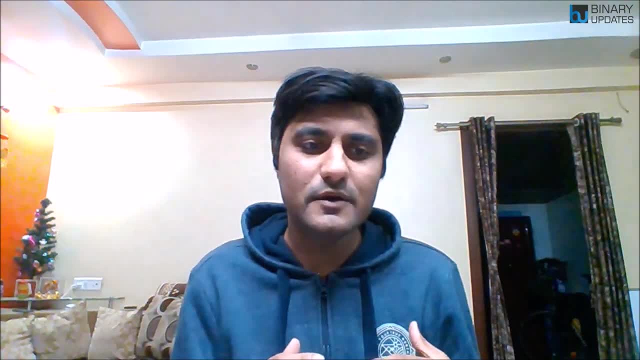 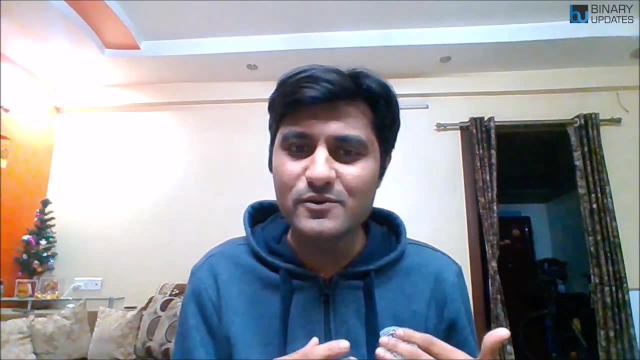 okay, it's more of a design job. and Then you also have to have a curiosity: how the Electronic component works, how the electronic things works. If you don't know those things, if you really don't like it, then it will be very difficult to become a very good. 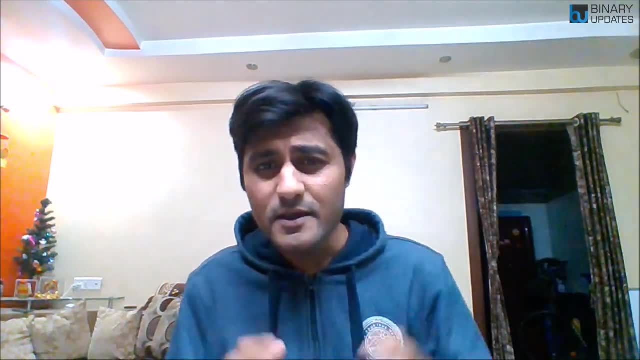 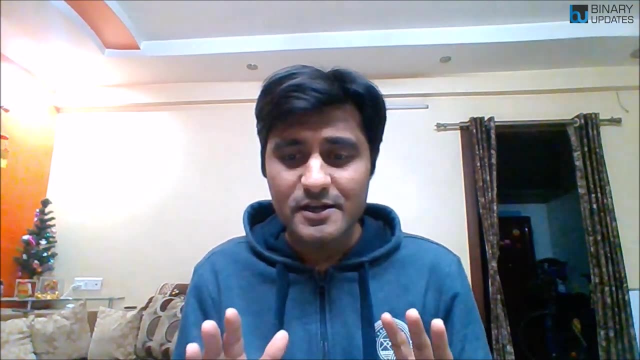 I mean, I'm just talking about a top-notch hardware developer. Okay, there are a lot of people they worked in the embedded hardware side but they just design a socket boards. They are not very good at, you know, simulating that socket, understanding how much current is flowing through every. 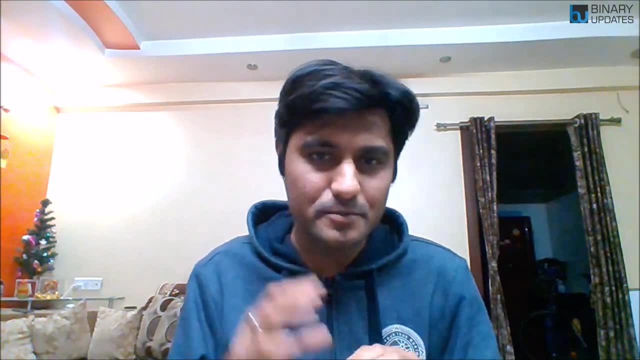 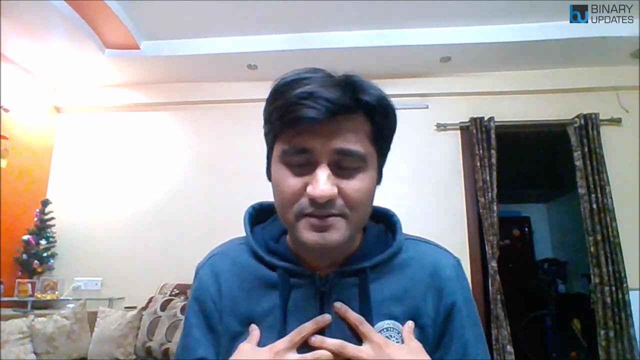 resistor and what is the impact of the capacitors and how the transformer, optocoupler and relay and all other things works. but If you, if you really don't like electronics by your heart, Okay, just like a designing, like a fashion designing for designing clothing. if you don't like that way. 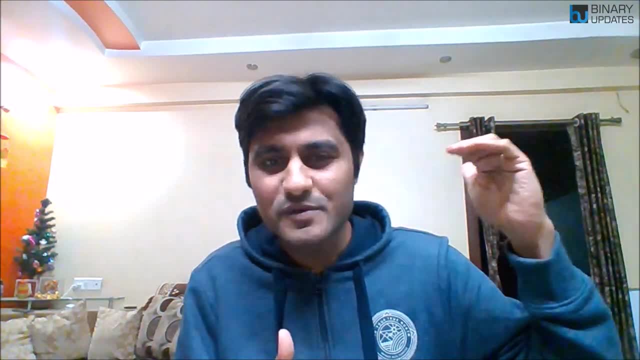 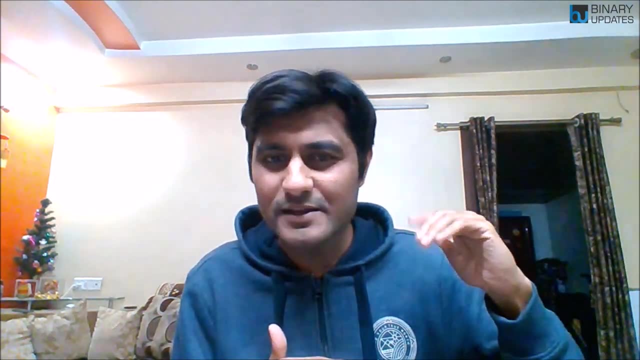 Electronics components, then it's very difficult to achieve the the highest results by becoming an embedded hardware engineer. So if you really wanted to go for it, if you love electronics, then you rather have to look for embedded hardware development. Yes, of course there needs a little bit. 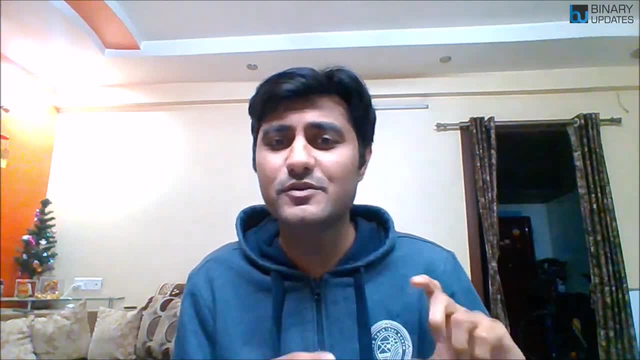 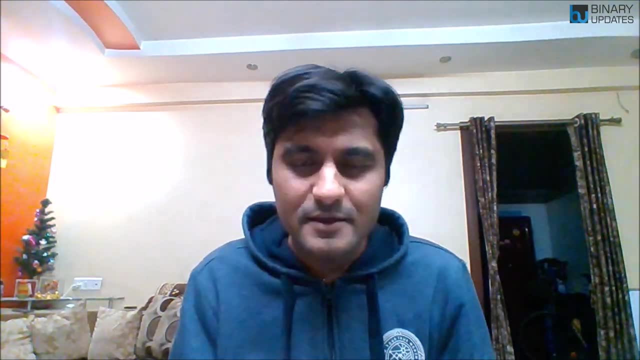 programming you must know in order to excel in that career. because if you Just design the hardware, if you cannot able to test it, troubleshoot it or write a software for making some small test, Then it would be very difficult to reach at the top to get the high paid job. 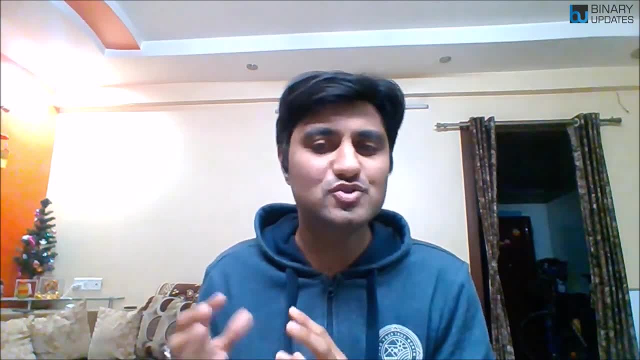 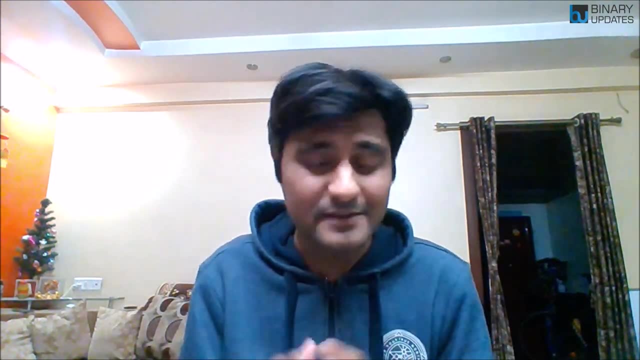 Now the other side of the game is embedded software site in embedded software developer, If you really wanted to prepare yourself for embedded software developer, because they're highly paid, at least in India. I have seen and even I studied in Europe, So I know they are much demanded profession, embedded software developer. 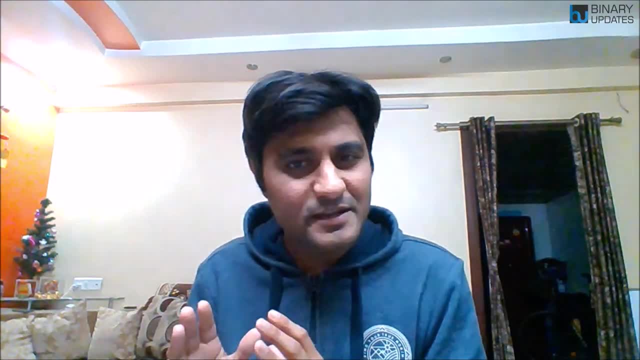 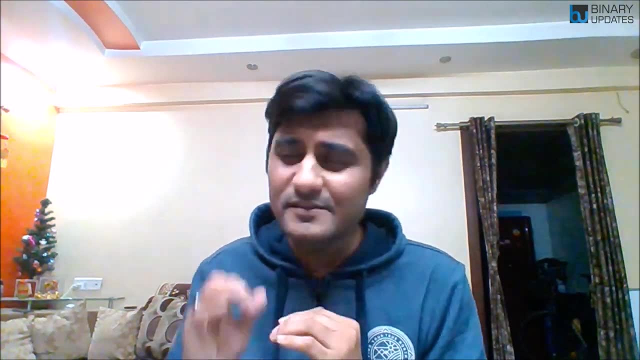 Okay. so if you, if you want to prepare for You, have to be very good at C programming. C programming is the basics. If you know the assembly programming, Then it's the cherry on the cake, but C is the basic. you must know C apart from C. 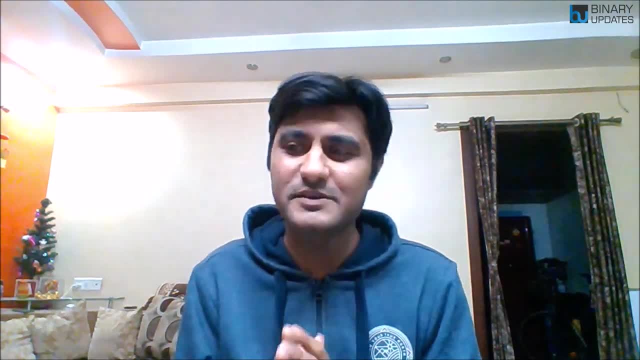 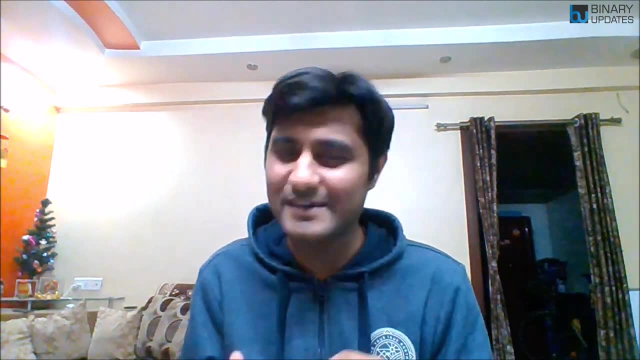 You should have to know the Python. Okay, it's good if you know Python, but it's not like you must know. It's not really like that. If you, if you, are very good at C programming, that's really great. If you know C++, then it's just a great. 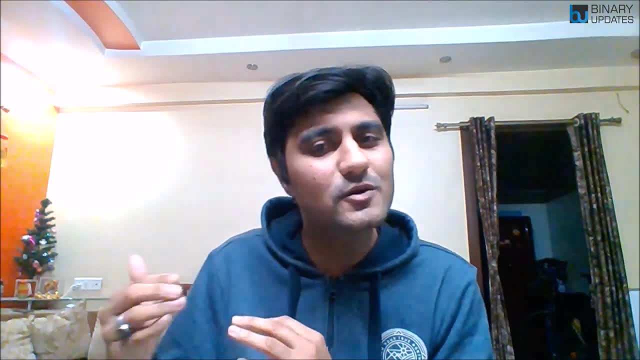 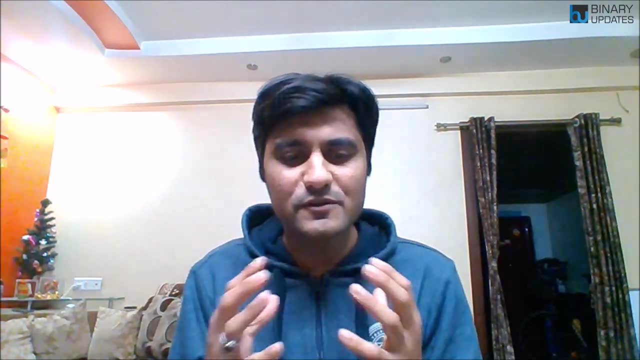 It's another like a cherry on a cake because you really excel very quickly. Anyway, someday you have to move from C to C++ And build a really complex application. But as a beginner, if you really wanted to start as a, you know That- like a graduate training engineer or junior engineer or the fresher in the embedded systems. 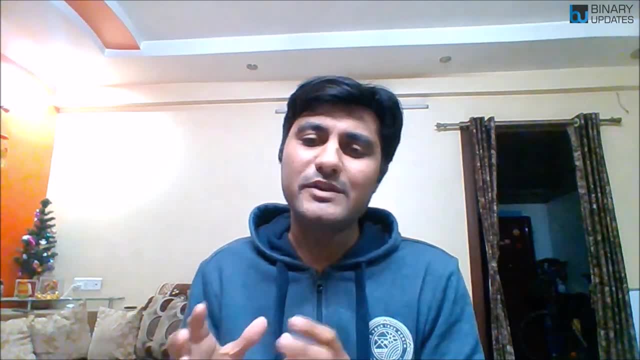 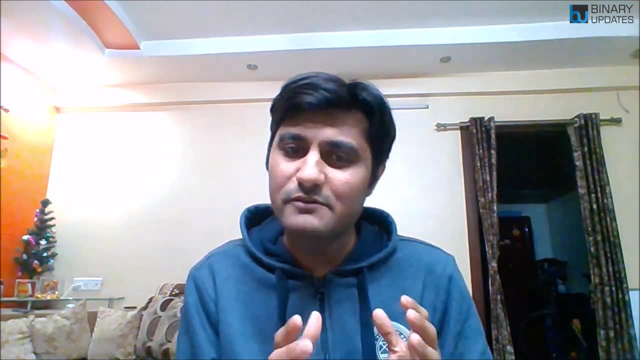 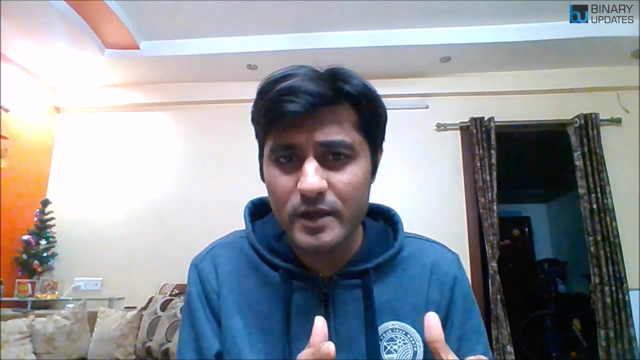 Then you must know C programming now when you write, When you become an embedded software developer, then only knowing C is not enough. You must have to have a love for hardware as well, Especially the low, low level architecture. I can say. I would rather put it this way: 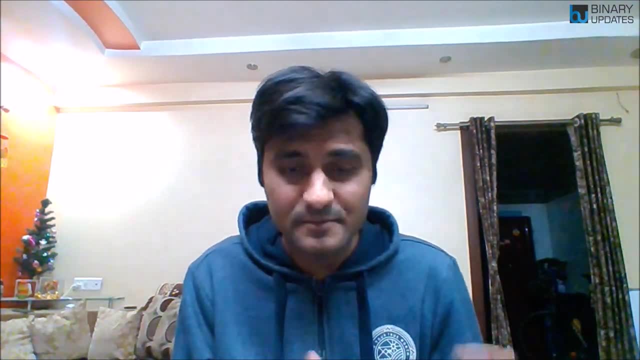 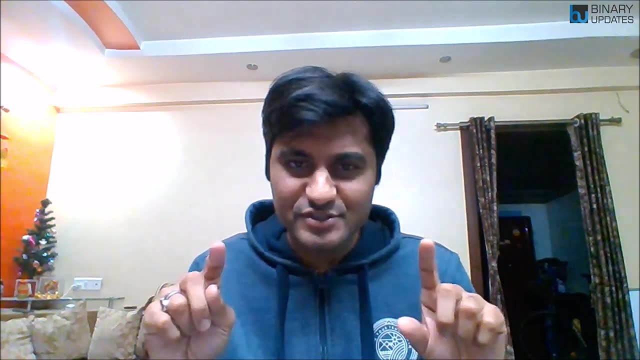 You must have to be good at like an operating system concept, because all the programming that you do using C++ is basically accessing the registers. Okay, so you must know the architecture of the chip, like an ARM architecture, Intel architecture, AMD, free scale. So there are a lot of architectures in embedded systems. 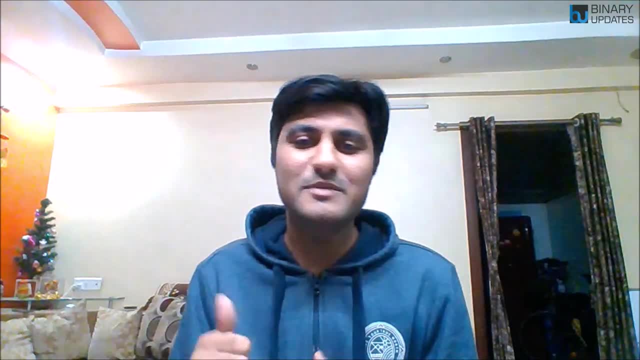 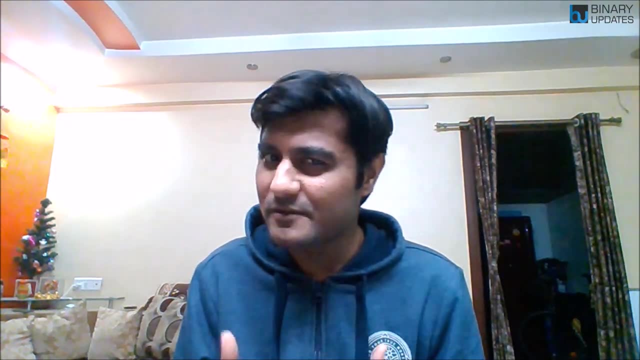 I mean, you don't have to learn everything by the way in the beginning. you can make one or two chips. I would rather recommend to go for a VR. That's the best architecture, very easy to start off because it's just a 8-bit microcontroller, but you have to be very good at C, That's. 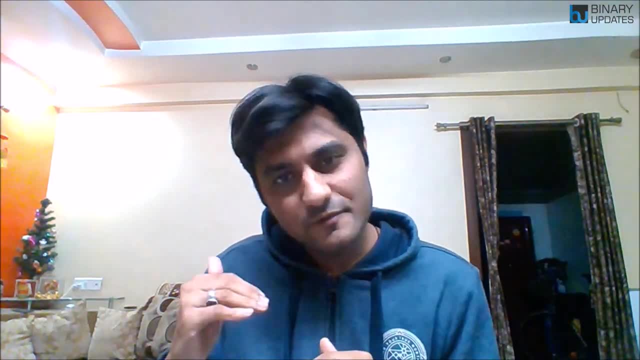 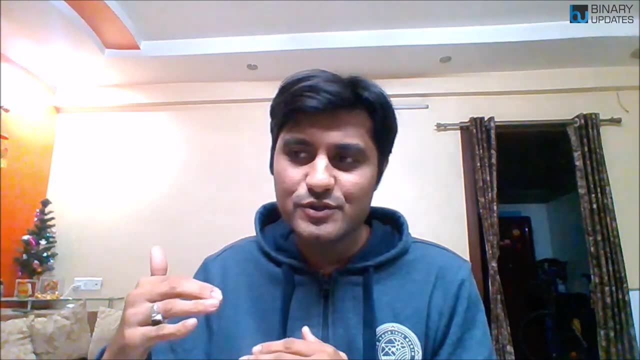 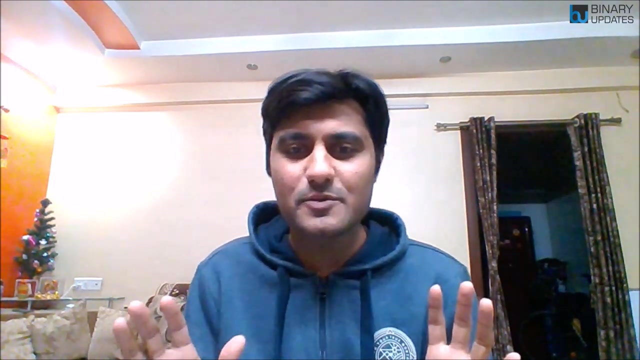 that's, that's the center point. and Going about that, you must know the operating system concept because someday In the embedded software development you will be getting a project working where you must have to know embedded Linux right, because you might see a lot of products around you maybe. 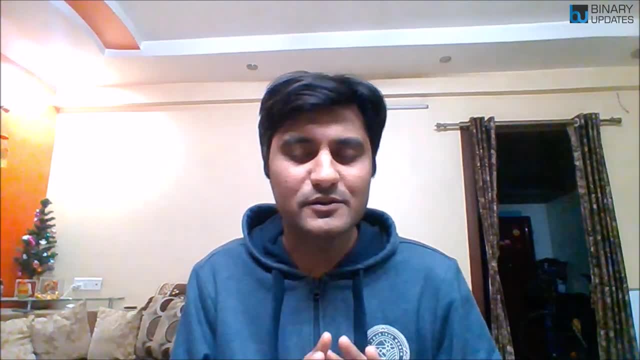 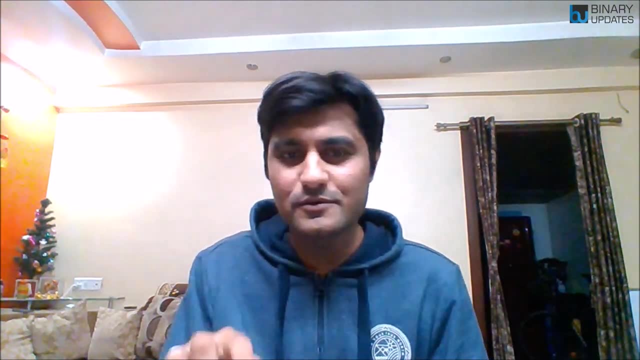 the touchscreen in in your car and maybe in your watch machines or maybe in a printer or maybe some kind of Healthcare devices. there are some touch screen So you press the button and something happens right. It's like a user interfaces that you make using a Linux GUI. 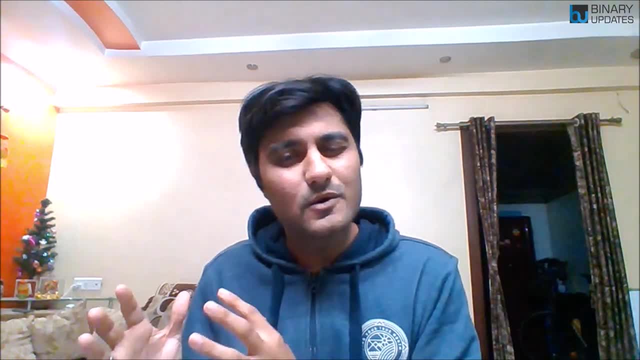 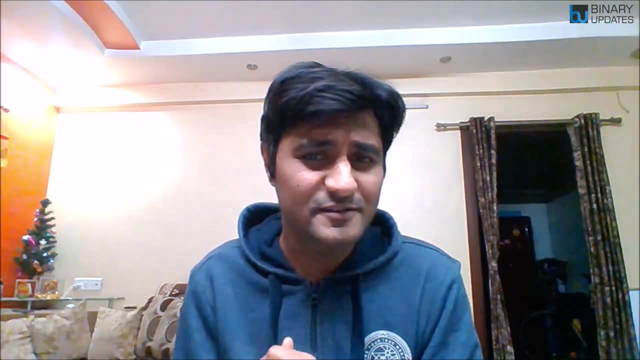 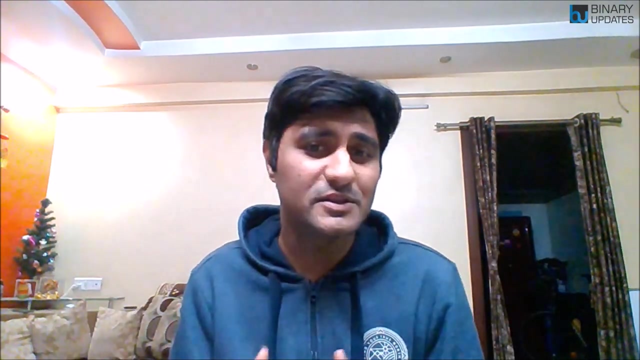 And so you, you also have to know a Linux along with the C programming So it could be like a kernel or device driver development and something like this. We're gonna talk little more detail about this, old things about embedded hardware landscape and embedded software Landscape in the future lessons if you really want to get start of as an embedded system engineer. 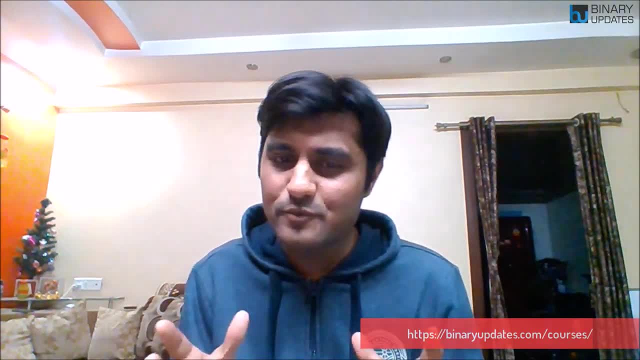 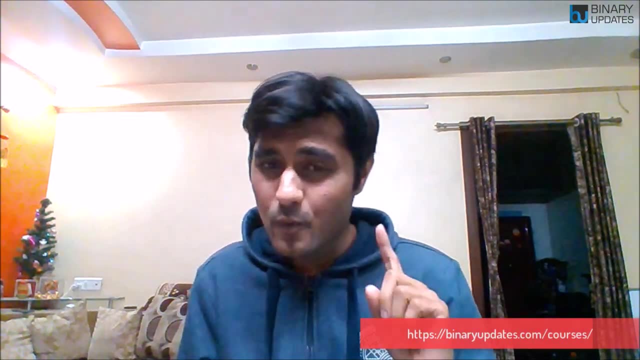 Then check out the link in a video descriptions. I do have provided some causes in the binary updatescom and I would really be happy to help you to get start of your journey Into embedded system. one thing you never have to forget is if you really want to be an embedded engineer. 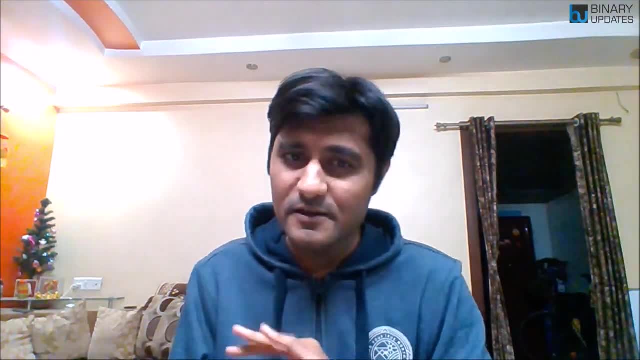 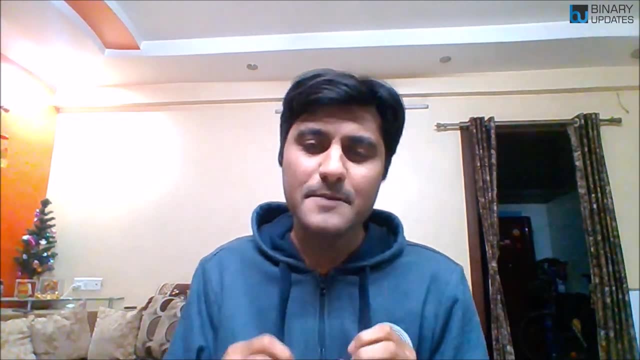 Get used to with a failure. a lot of projects, you're gonna make it. a lot of socket board You will design. a lot of software you're gonna write they would never able to perform as per your expectations. but you take this project which doesn't perform to your expectations and 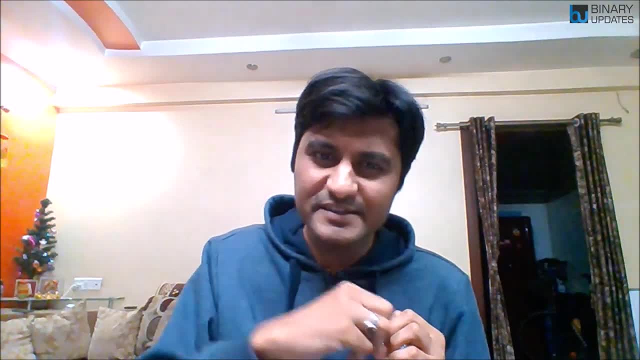 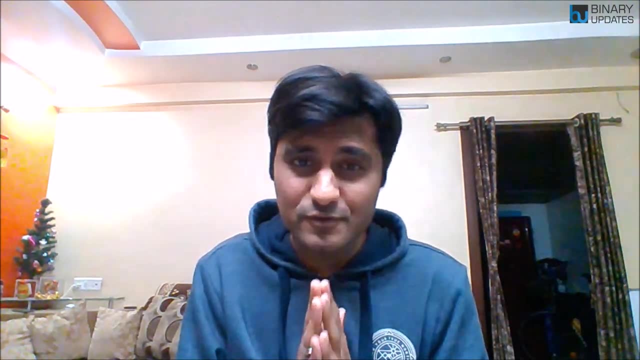 you know you just You just scale it to the, to the point where you make the software to work with the hardware, So You don't have to scare to make a mistakes. This is a field where you make a mistakes, you learn and then you move on. 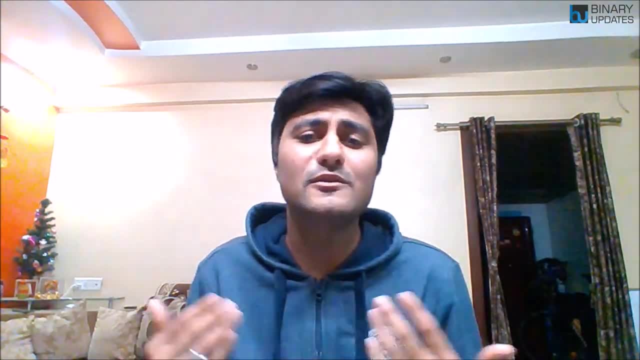 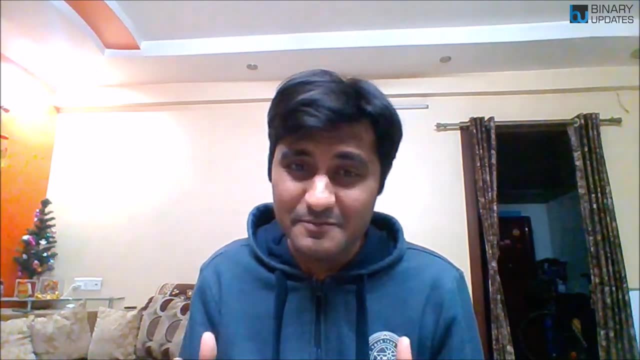 That's how the embedded system engineers are made. I, in my life, have made a lot of mistakes. I still remember when I was doing my bachelor studies I was trying to make a radio receiver and, believe me, it took me a long time. I mean almost like one and a half year or something. It was like 2009 back in. 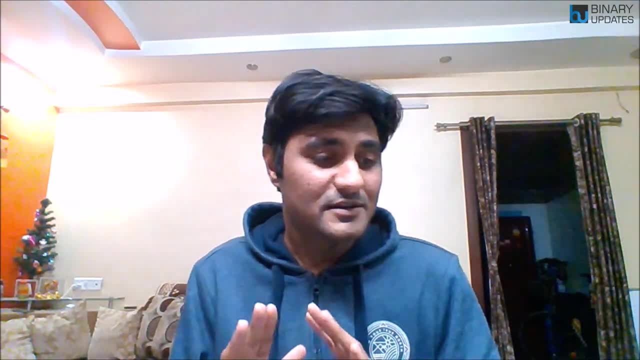 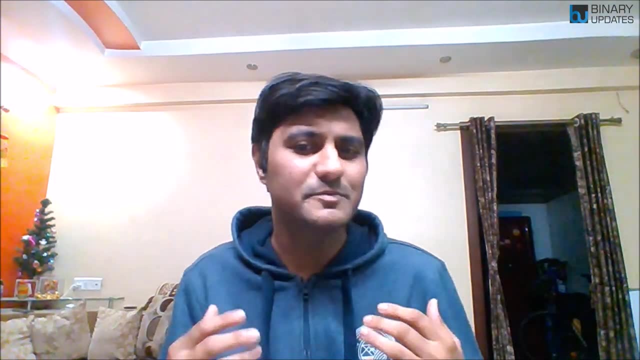 Time when I was very young and I was new, there were not much of a help online, So Really, you just have to get used to with a failure, a lot of projects You're gonna build which doesn't work, but every project will teach you. so this is how it is. 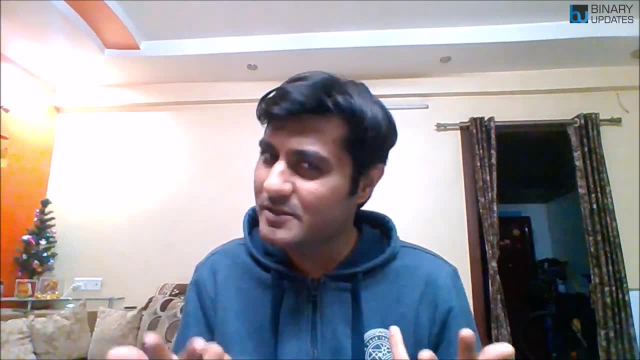 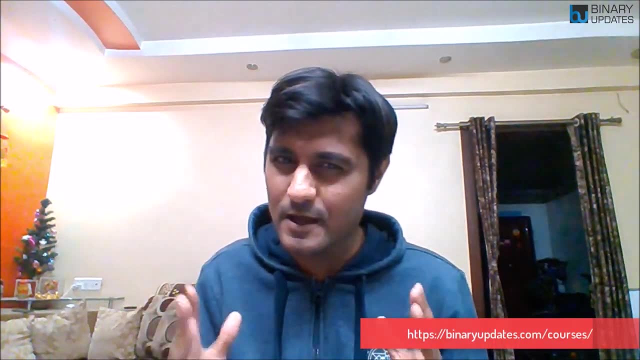 I mean, you can build the projects and you can excel. if you want to build a project with me, as I said, check out the link in the video description and Get in touch with me and we'll see how best I can help you. Thank you very much for video. And we'll see us into the next lesson. Bye, Bye.